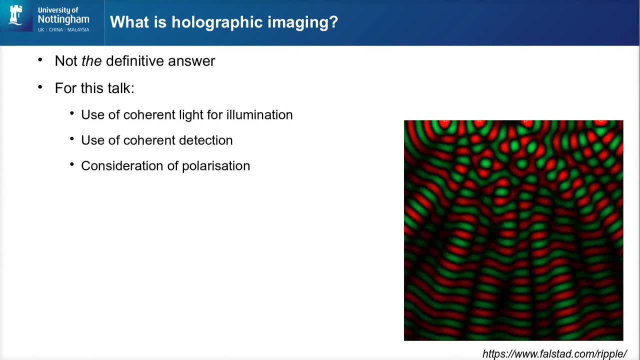 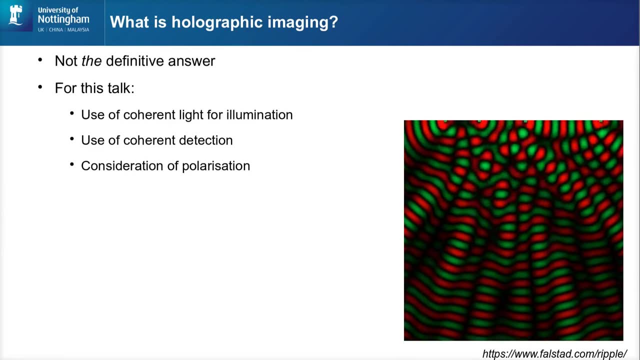 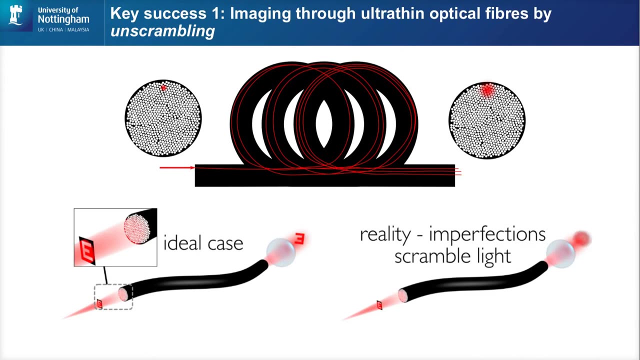 here's a simple demonstration of the kind of complex patterns you can get when you just got four sources that are beating together at different spacings. so that's kind of the general idea of what holographic imaging really means. it's all about diffraction and interference of wave fronts. So now I'm 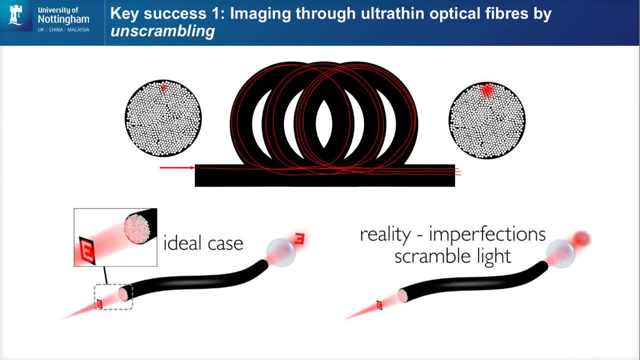 going to talk about the sort of three key successes that I've identified in this area. So one really important thing for holographic imaging is that it has recently enabled the ability to image through our optical fibers- ultra-thin optical fibers, despite the fact that they scramble light. So I've given here 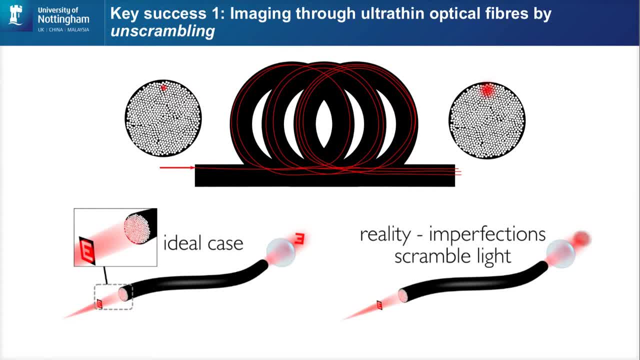 a sort of intuitive example, which is the example of a multicore optical fiber that's commonly used in medical imaging. what happens is you send light down one core, but actually it doesn't stay confined to that very well all the time. so when you're sending light down to one core, you do not get what you're. 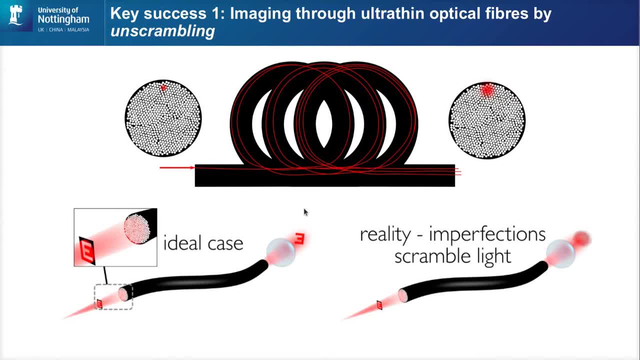 against the other end. it's spread out a bit. So this kind of spreading out also includes phase shifts between these different paths down the fiber, and so ideally for perfect fiber, you could just coherently image straight through and it would just transport the optical field from here to here. 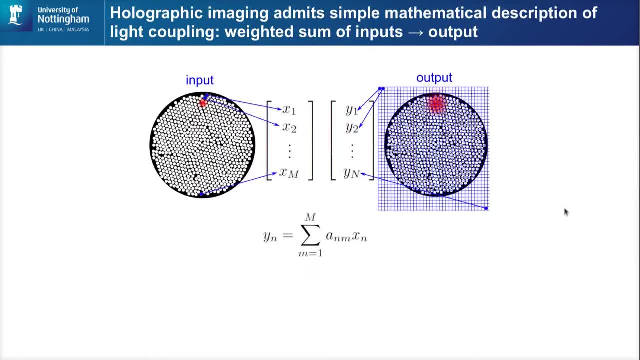 but in reality these imperfections mean that this is scrambled. So the use of holographic imaging, which effectively measures the phase of the wavefront, emits a very simple model of this scrambling, which I'll just kind of briefly go over here, which is that you can consider every single point on the input. 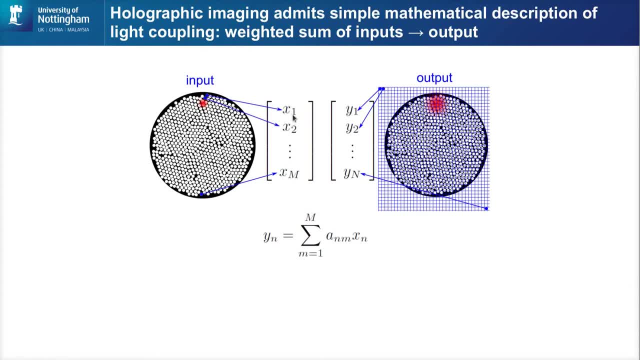 to be denoted by an element in a vector and every single point on the output, you know, perhaps discretized on a camera, and a rectangular grid here to be denoted by another vector. y Well, if you're using holographic imaging, then the relationship between the 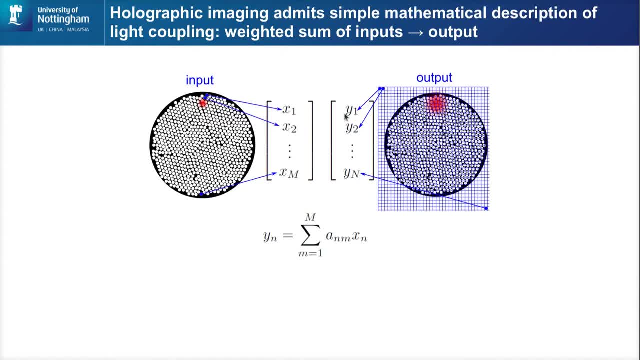 y and x is just linear, so each y is just a weighted sum of all possible input values. okay, so which we can write like this: and so if we then relate that together, what we can find is that each single y has a different set of weights based on how it depends on the inputs, and so we can actually write that. 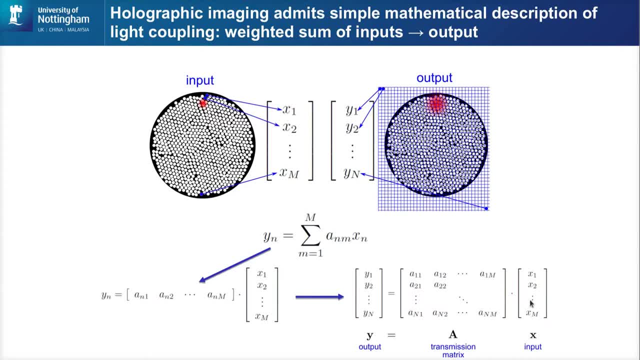 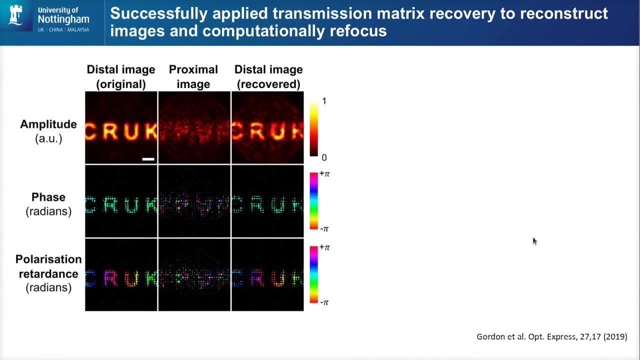 as a matrix. So we have an input vector times a matrix times an output vector. it's perfectly linear And this linearity means that any distorted output that you get, like this middle row here, you know you can invert that matrix and get a recovered input over here. 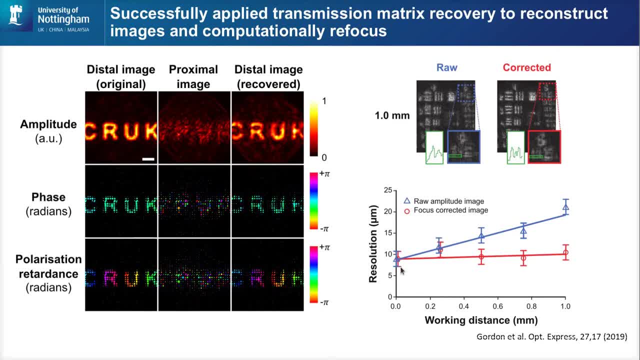 Furthermore, because you can recover this image, because it's holographic imaging, you get not only the amplitude but you also get the phase information, which means you get the full wavefront, and so you can do correction for you know, for defocus, or here's an example from a recent paper in mind which showed that we can move the 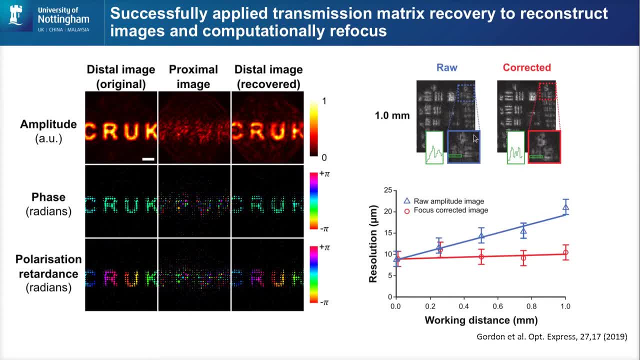 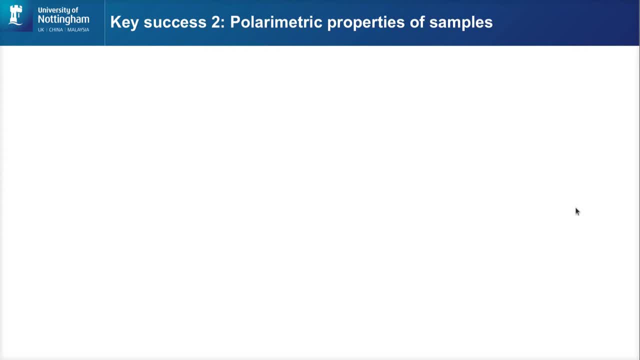 sample a millimeter away from the end of the fiber and using this phase information, we can correct for the defocus. So the second key success, I think, is that if you're using this holographic approach and you're really being forced to consider the phase, 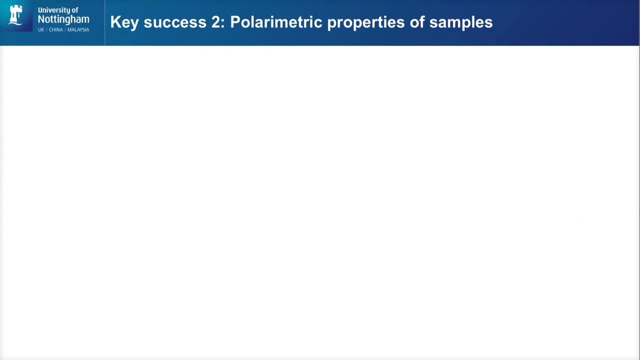 of the wavefront. well then, it's not too big a jump to also consider the polarization of the wavefront. you simply have to consider the phase, you know for two different, split the output using a beam splitter or something like that, and then consider the phase in both angles. 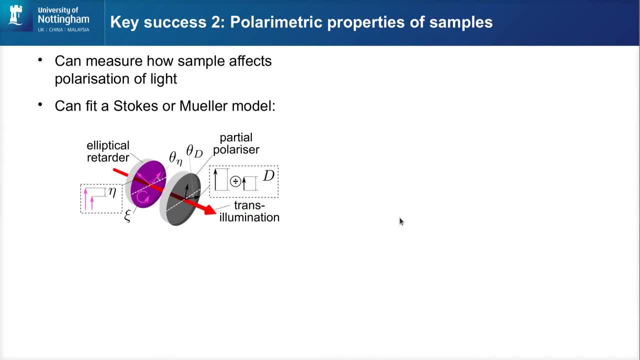 So using this holographic imaging we can then fit a model of our sample. so here I've used an elliptical retarder followed by a partial polarizer, and then you can use Stokes or Mueller polarimetry to actually fit this model to the data you get. And here's an example where I've done. 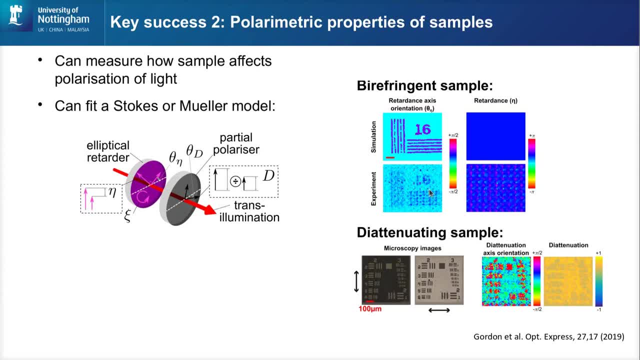 that through an optical fiber and I've managed to fit. you know, I've got here four different polarization parameters that I've managed to recover from the samples, So that's really nice and that brings you extra information that you couldn't normally get. you know, retardance axis, di-attenuation. 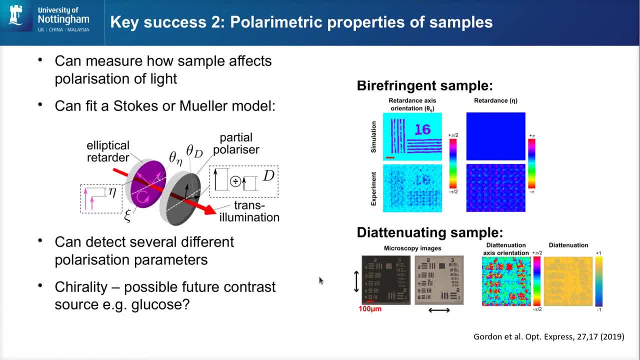 axis, but I think there's a lot more to be done in this area, because there are things that this can detect that I've got here, such as chirality, which could potentially be used for detecting things like glucose or other chiral molecules. So I think there is a lot to be explored in this area. 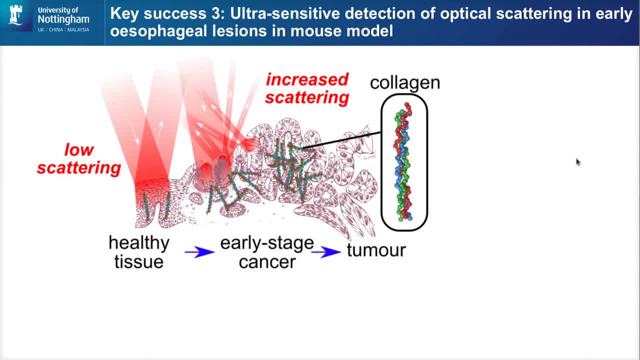 And a third success of holographic imaging is the ultra-sensitive detection of optical scattering. So the kind of concept being that a very, very early stage cancer, you get these you know, very disordered microstructure that starts to form on a very small scale, both from the cell structure and also 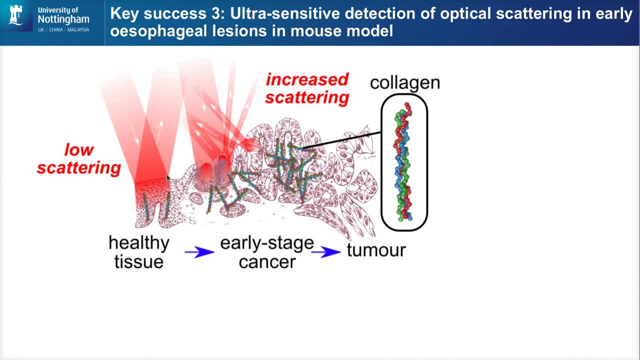 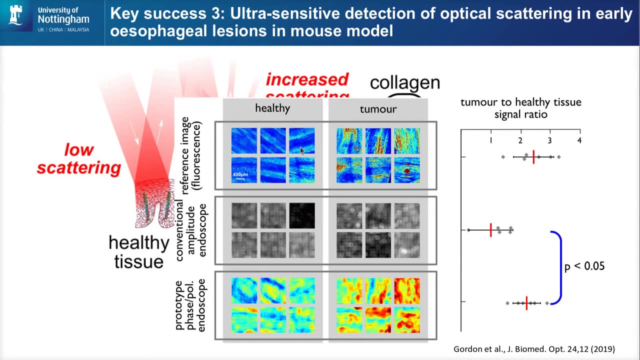 from these dense networks of collagen and this reflects a bit more differently. This is more of a specular reflection and this is more like a sort of diffuse reflection here and I actually we were actually able to show that when we image some mouse esophageal tissue- here's some healthy on the left and 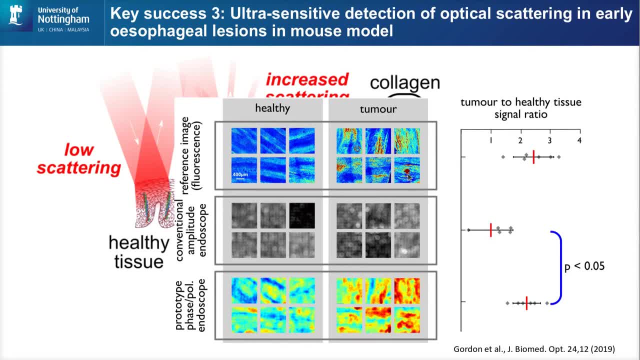 here's some tumors on the right. This is a depi stain, so we can see increased density of cell nuclei. using the optical phase information and looking at the deform, the level of deformity of the wavefront, we can actually see improved contrast using the phase information compared to just using the. 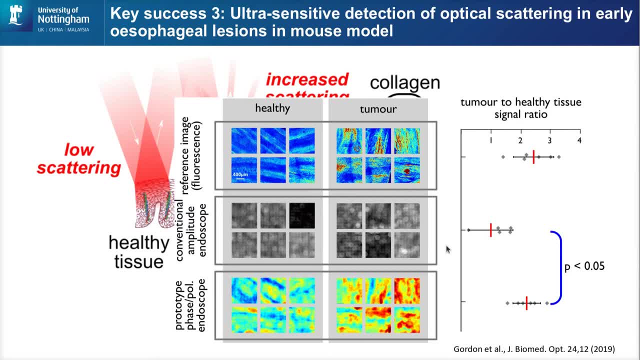 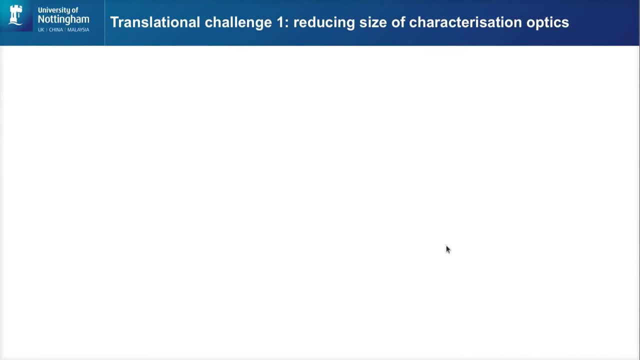 aperture information alone. So those are kind of three successes, recent successes that I've identified about holographic imaging. So now I'm just going to talk a bit about some of the translational challenges. You know why isn't this technology being widely used in clinic? Well, without going into too much detail, 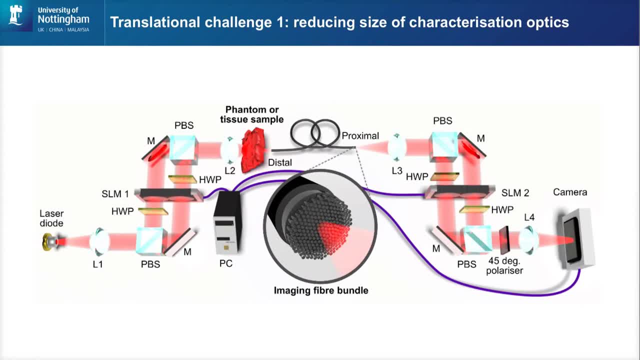 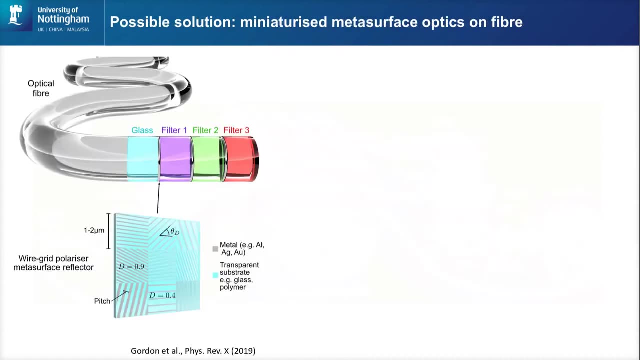 here's the optical system that I use for many of the results that I showed before. Now the problem is that to translate this, a person would need to swallow all that equipment now, which, I must say, is rather large. so reducing the size of this is a key translational challenge and the way I'm planning to approach. 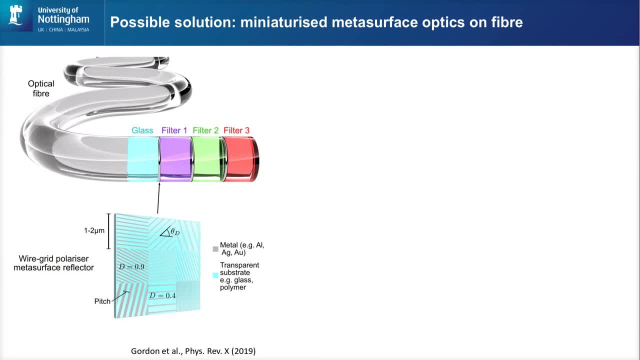 that is. you know if I propose to approach that is is to basically use miniaturized optics on the end of the fibre, particularly enabled by the use of metasurfaces. So here I've got this kind of stack with different filters and I've got metasurfaces in between, and by doing that you can actually effectively miniaturise a lot. 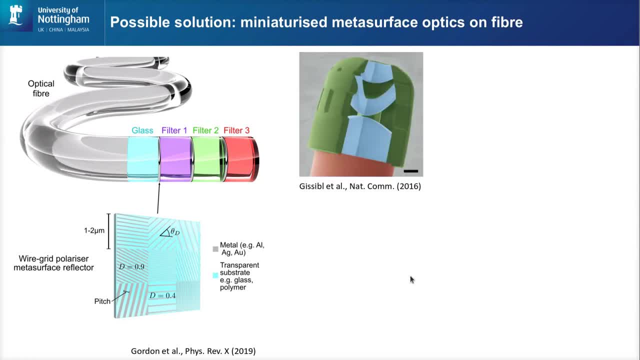 of the passive optics from the previous slide and stick it on the end of the fibre. You know, and so this is you know, something that other groups are working on too. so people using two photon techniques and also, you know, standard electromimithography techniques to make nanostructures. 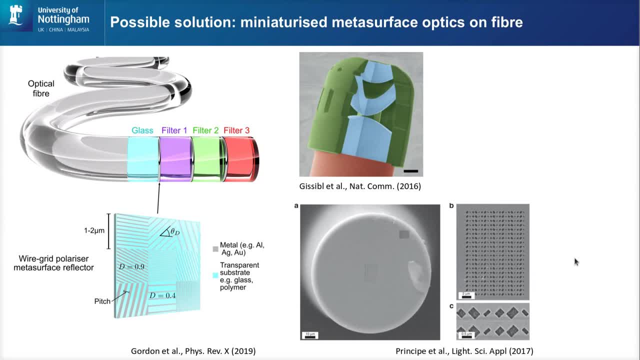 on the end of fibre. So I think there's a lot of potential there and I think, you know, one really exciting potential of being able to get to this level of miniaturisation is the potential to actually put all of this advanced optics on the end of the fibre that can go through a needle. 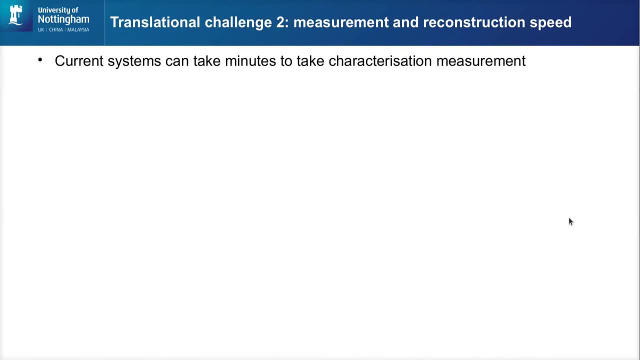 and then be inserted into the body. The second translational challenge is the measurement and reconstruction speed. So current systems can take minutes to take a characterisation measurement and this is challenging because you might have to take characterisation measurements every time the fibre is bent because it upsets that transmission metric I talked about earlier. 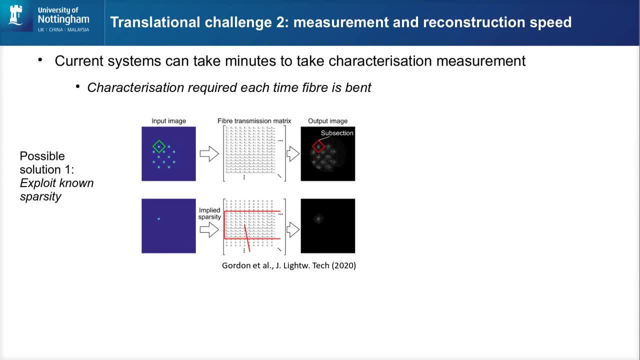 So there are some possible solutions to this as well. One is to exploit known sparsity. It's in the case of multicore fibre. that simply means sending multiple beams down. This has been generalised by some colleagues of mine at the University of Exeter into actually a way of sort of doing the minimum. 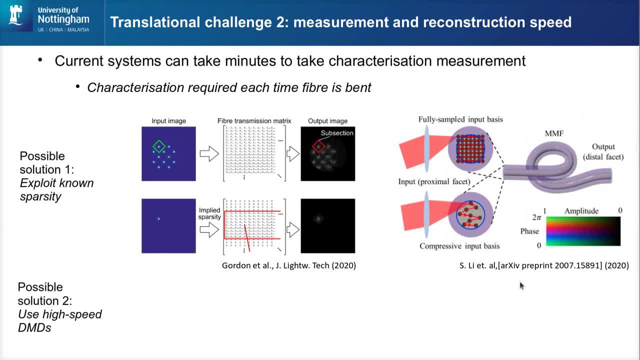 possible number of measurements for a multi-mode fibre, And you know, another way of speeding this up is to move from using spatial light modulator devices with liquid crystals that are quite slow to using high speed digital mirror micro devices, and there are people working on that too, So it's not just the characterisation. 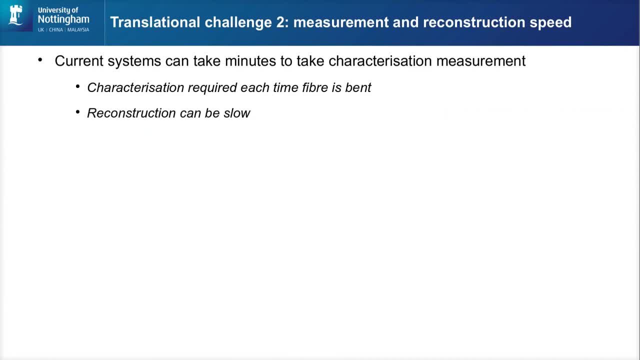 time that needs speeding up. The reconstruction time, which is taking these characterisation measurements and recovering images, can also be a bit slow. So one solution to that that is promising for the future is to actually use pre-trained neural networks. So you train them on a huge data set of input and output things and then, once it's been trained, it can very quickly. 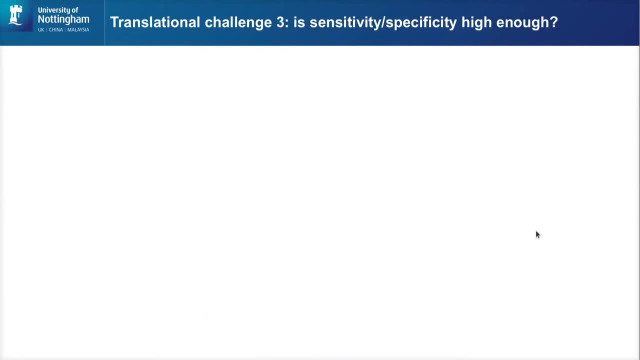 do the recovery for you. So I guess the final major translational challenge is: is the sensitivity and specificity high enough of this holographic imaging technique- And this is a difficult question because you know you can ask this really of any approach that's not yet been clinically validated- and it 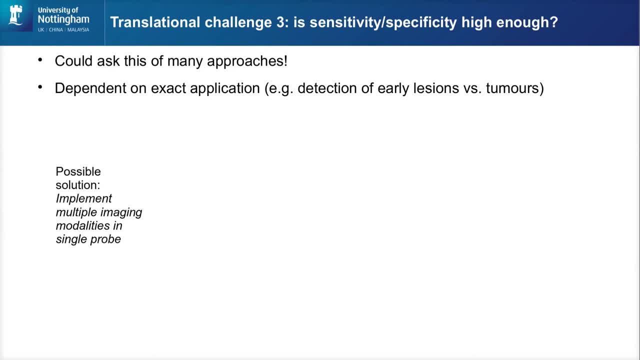 will depend on the exact application, But for this particular technology, the way I like to look at it, is one possible solution, And that's the holographic imaging technique. So I'm going to show you a little bit of my own personal experience with it. But the solution is to view holographic imaging as